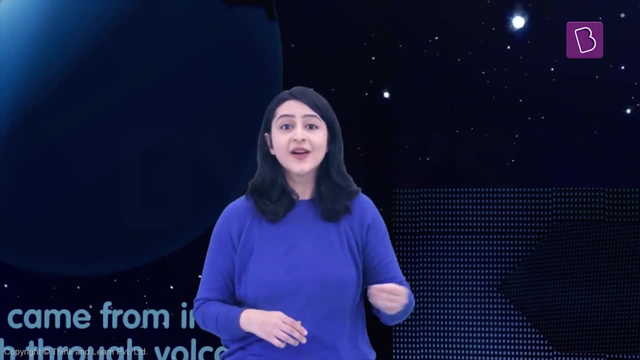 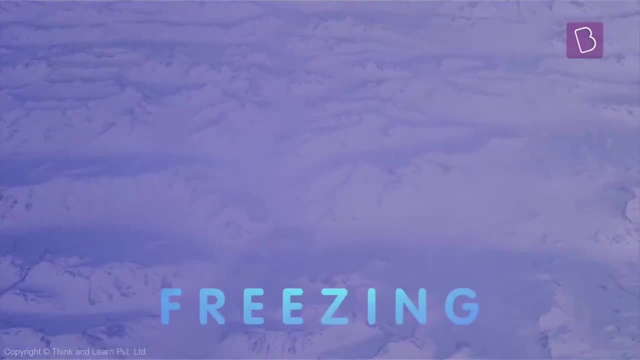 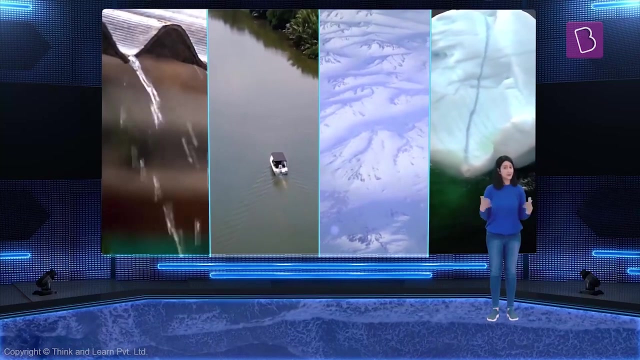 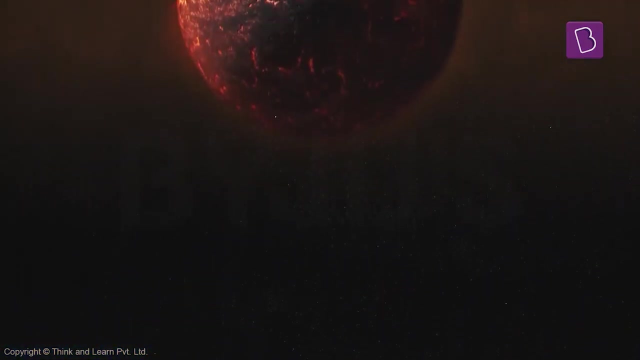 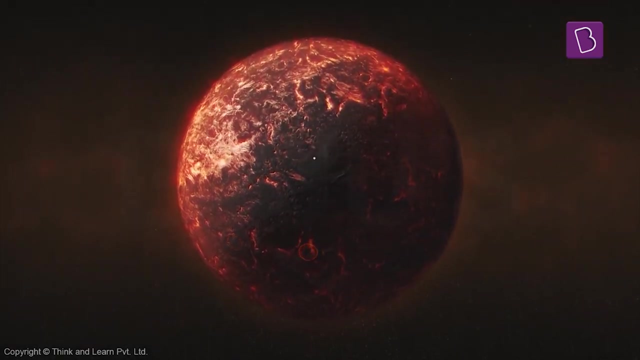 later, the same water is still around, Trickling, Flowing, Freezing And floating. So water has indeed lived a long life, but in different forms. Ancient Earth was fiery and fiery, But it was not only fiery and fiery, It was. 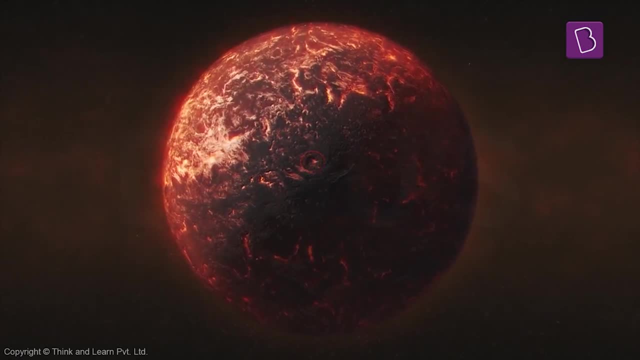 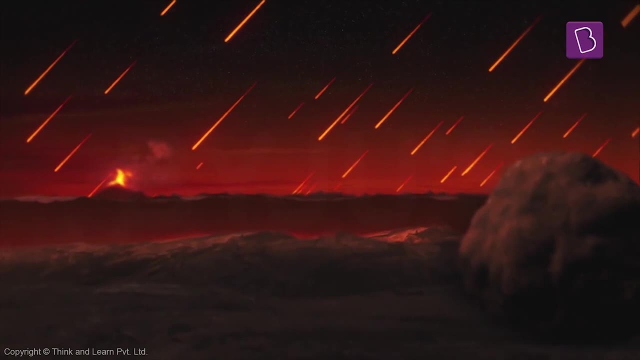 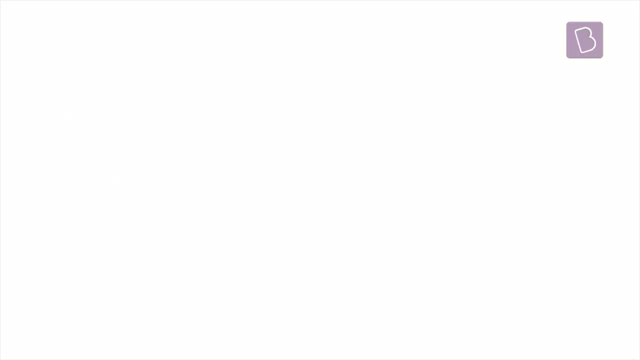 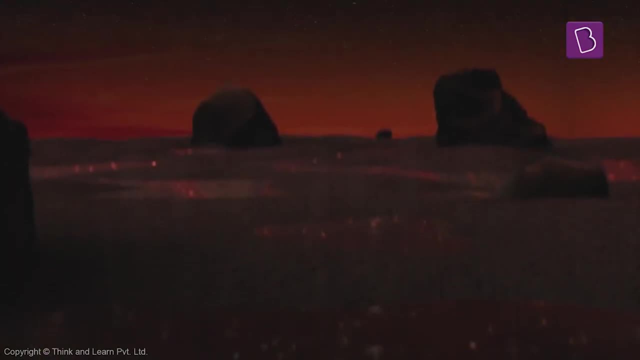 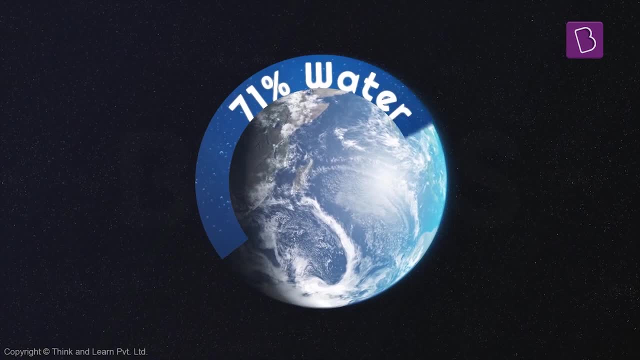 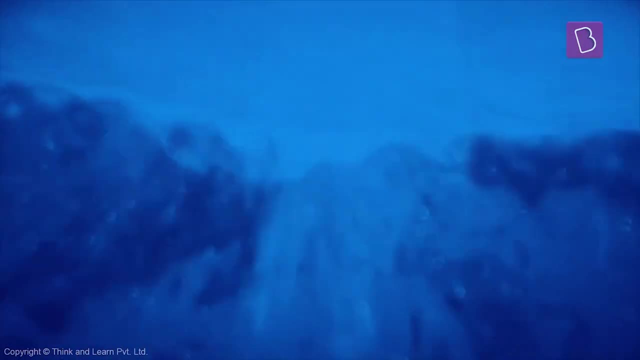 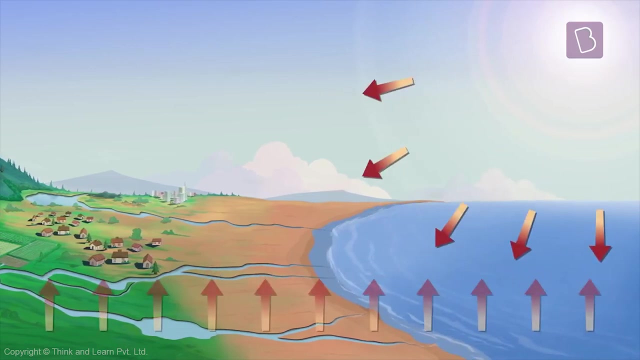 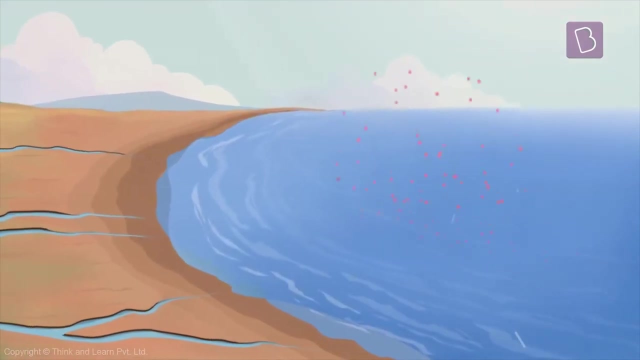 When you look at the surface of the earth, it is 71% water and the remaining 29% is land. The bright sun shines and heats up everything on the earth, water and land alike. When water gets heated up, water molecules absorb heat and move into the atmosphere as. 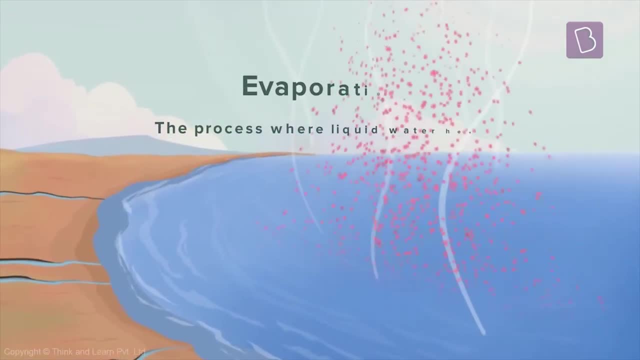 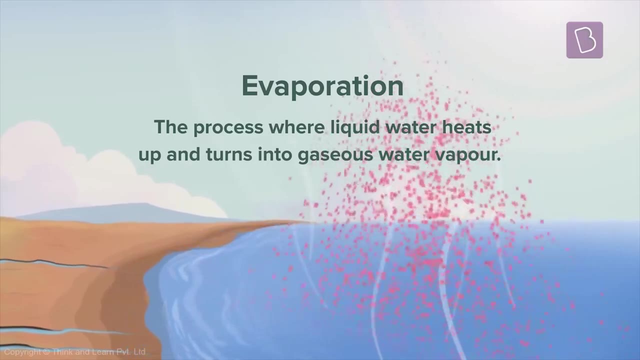 water vapour. This process, where liquid water heats up and turns into gaseous water vapour, is called evaporation. The vapour is the process of evaporation. The vapour is the process of evaporation. The vapour is the process of evaporation. 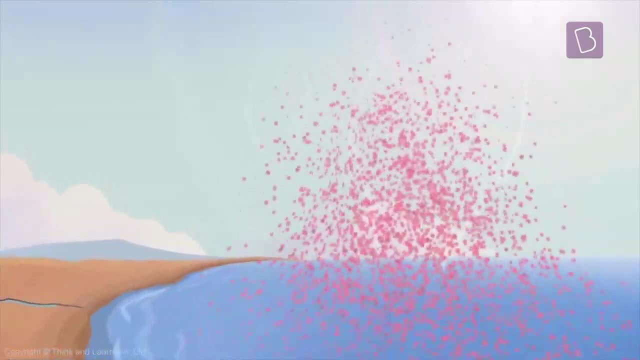 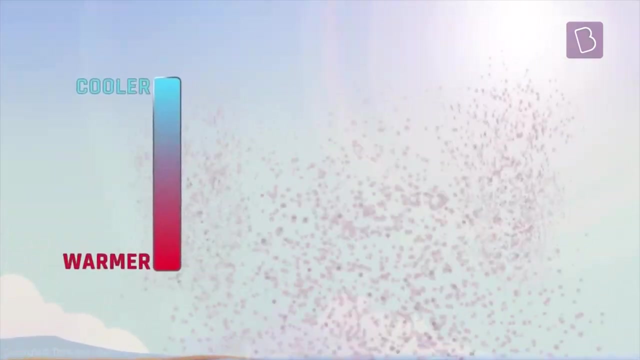 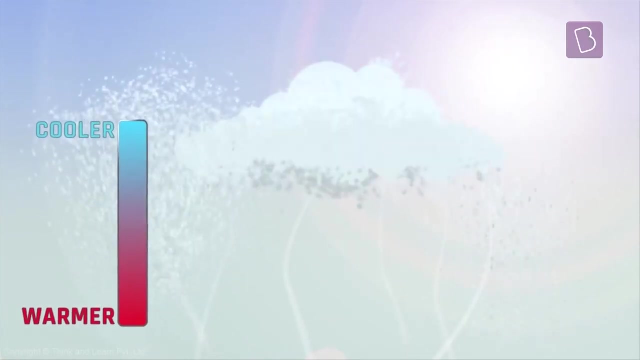 The vapour keeps moving upwards and soars high above the ground. In these higher regions of the atmosphere the temperature is really low, So the water vapour cools down in droplets and forms clouds, some going on to be tens of kilometres long. 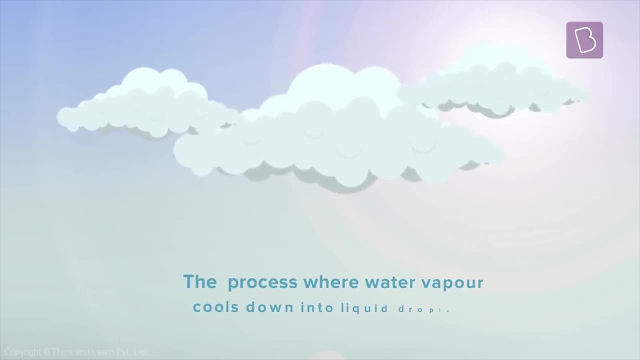 This process, where water vapour cools down into liquid water vapour, is called evaporation. In these lower regions of the atmosphere the temperature is really low, So the water vapour cools down into liquid water vapour is called condensation.